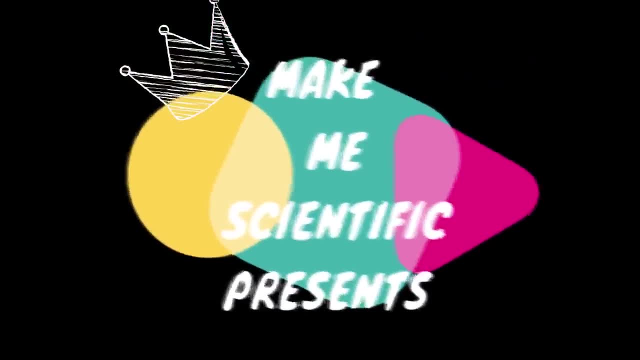 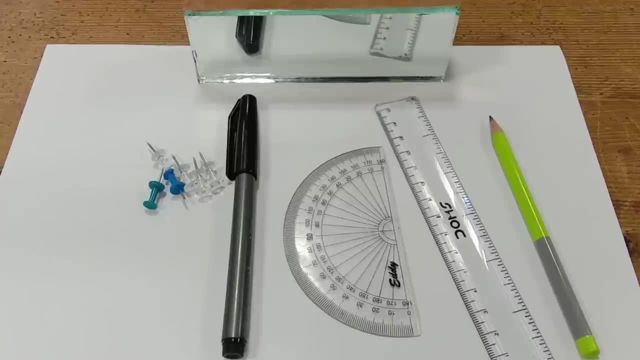 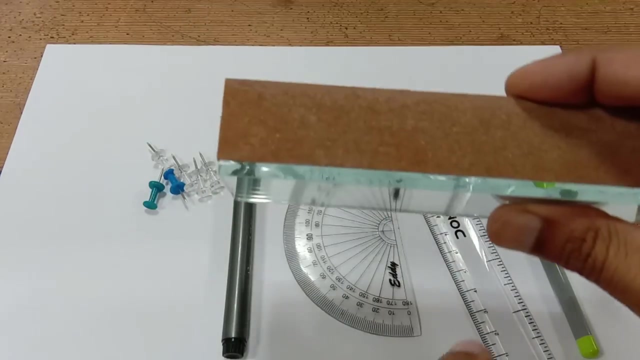 A simple experiment to prove the laws of reflection, that is, the angle of incidence is equal to the angle of reflection. So for that I require some basic stationary items, I require some softboard pins and I require a plane mirror. So this plane mirror is actually I am. I have attached a wooden 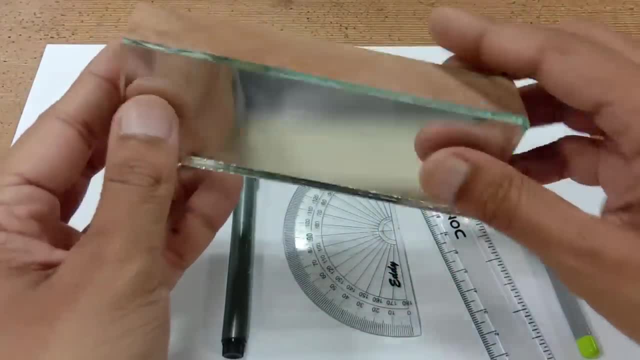 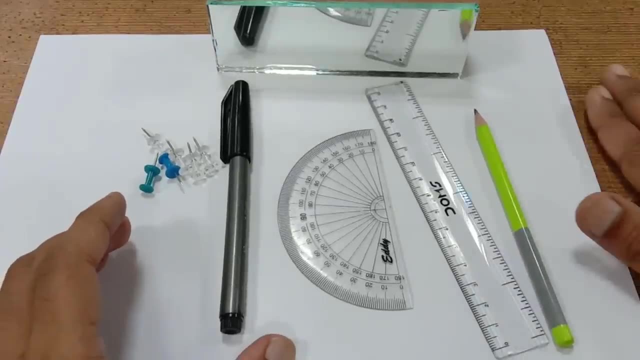 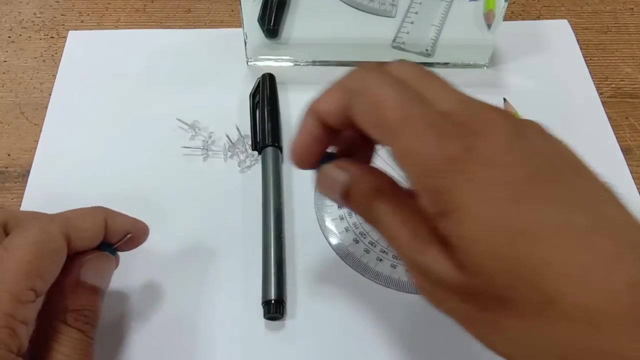 block at the back side of the plane mirror so that this mirror can stay upright right. I also require a wooden board on which I am doing the practical as well as I require a A4 size paper. Now what am I going to do is I am going to fix my A4 size paper so that it doesn't move during. 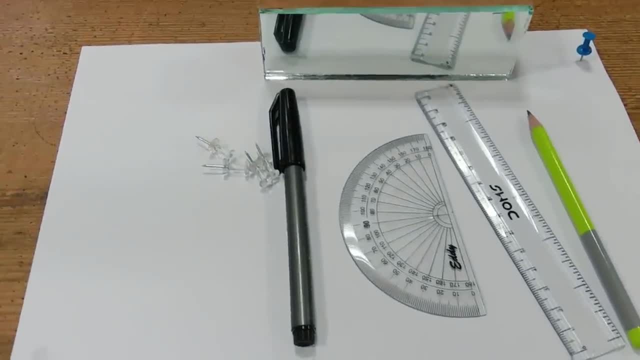 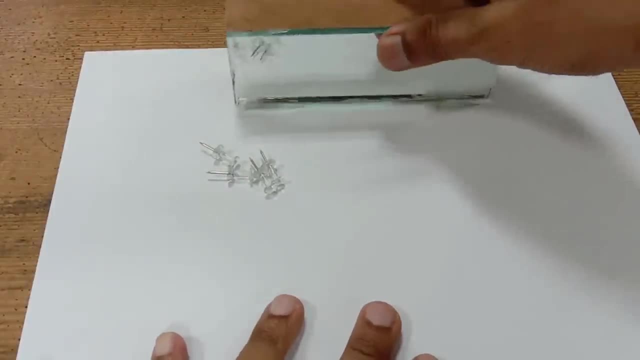 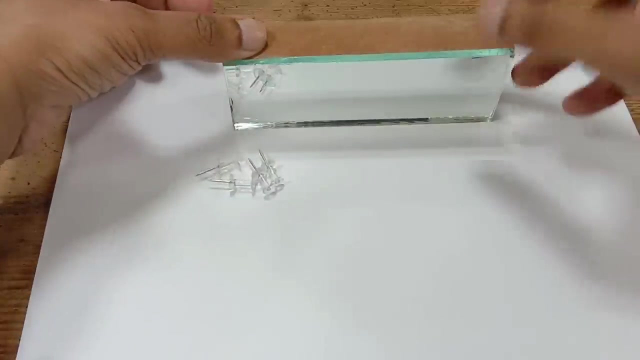 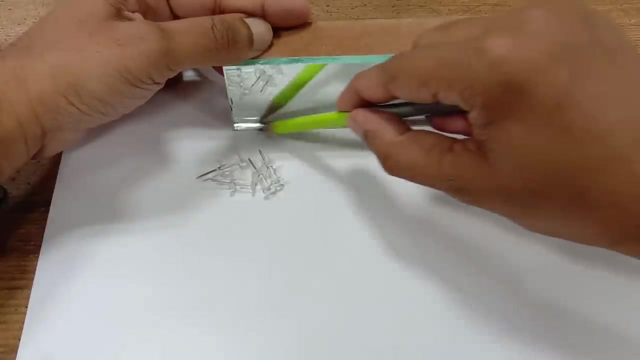 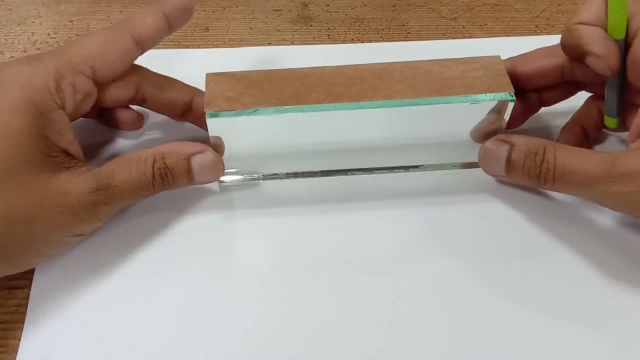 the entire experiment like this: Now let me remove these all things from here, And I am going to place a mirror somewhere over here and make sure that this mirror is kept straight, And then I am going to draw a straight line like this: Okay, So I will have to do it again. 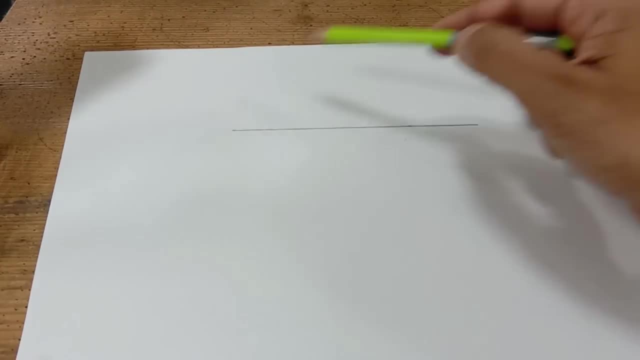 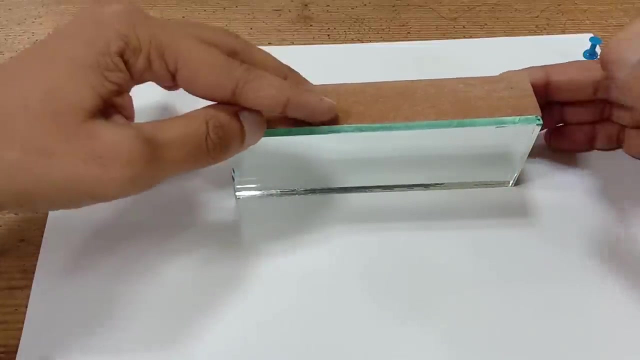 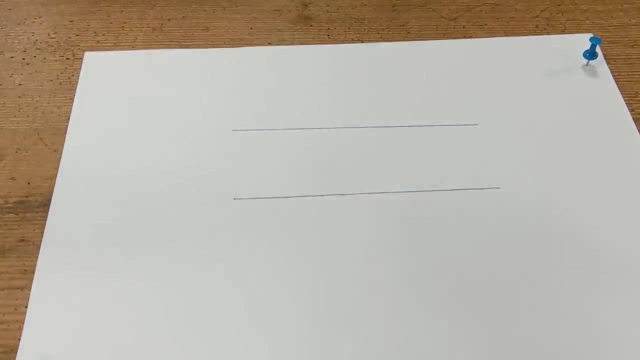 because, as you can see, the distance from here to here and the distance from here to here are not same, So let me do it again. Okay, This is my line that is ready, of the mirror. So this is basically my plane mirror and you are. 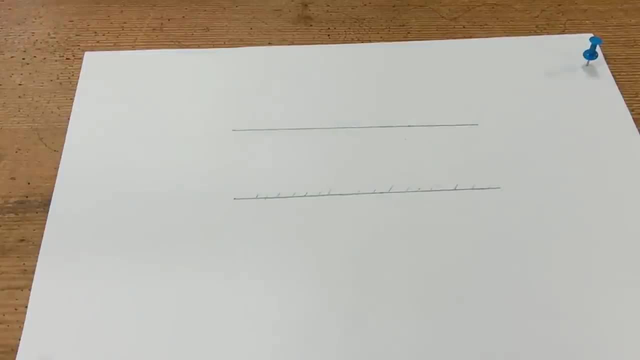 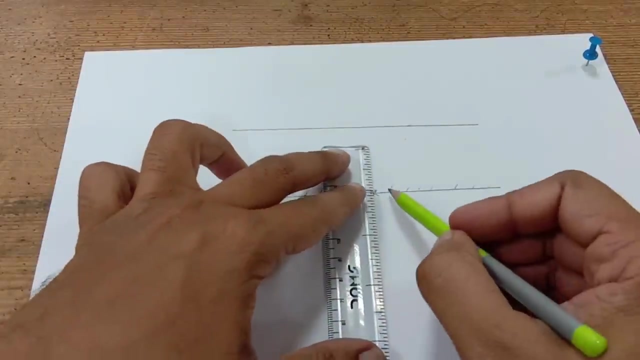 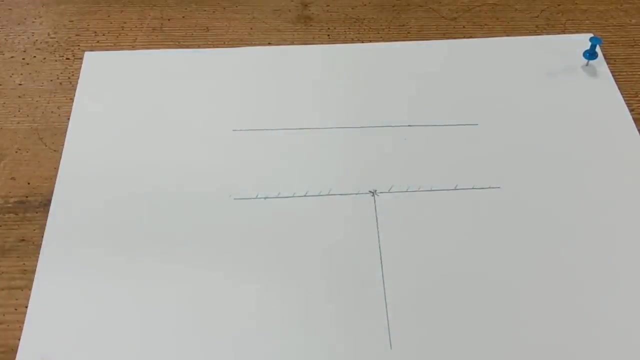 looking at this non-reflecting part, and this is the reflecting part right Now, at any one location, say at the middle, I am going to draw a perpendicular line, So this angle is 90 degree. Now I am going to place this mirror back again over here, not on this line. Now, let me. 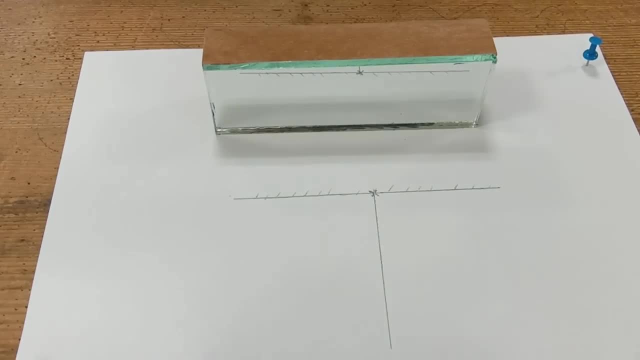 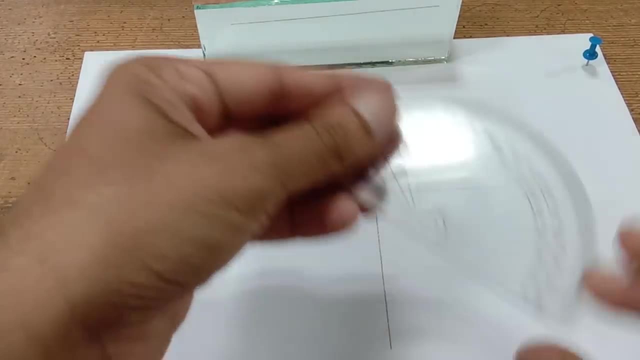 keep some angle of incidence. that is up to us. You can take it 30 degree, 40 degree, 60 degree, whatever you want. So this is my protector and the zero of the protector that I am going to keep it over here at this point like this. 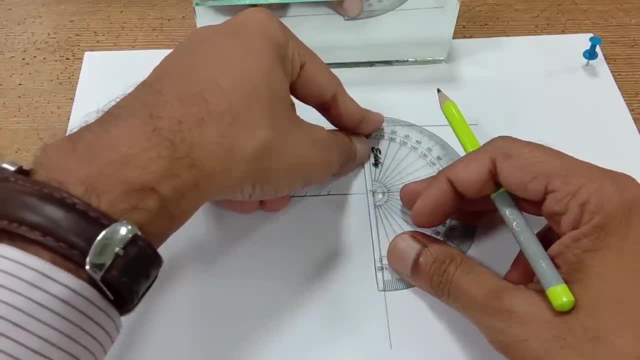 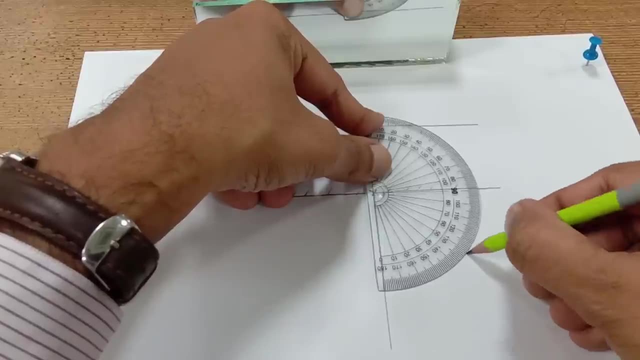 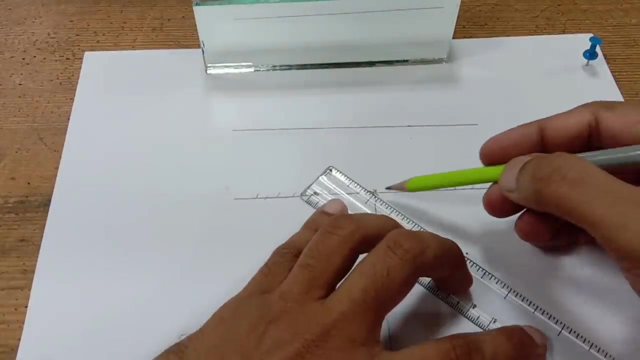 So this line is matching with this line. Let me make the angle of incidence. This is 0,, 10,, 20,, 30,, 40,, 50 degree. Fine, So let me make this angle of incidence 50 degree. So from here, 50 degree. let me join these two points. 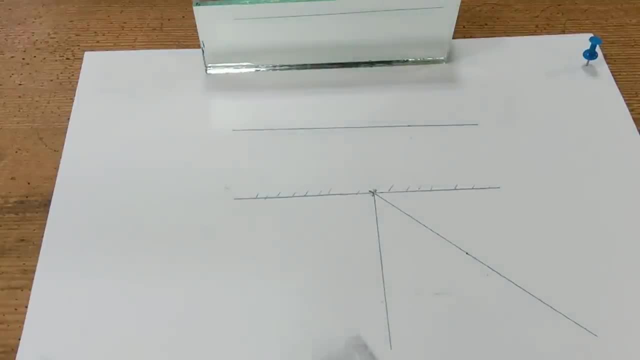 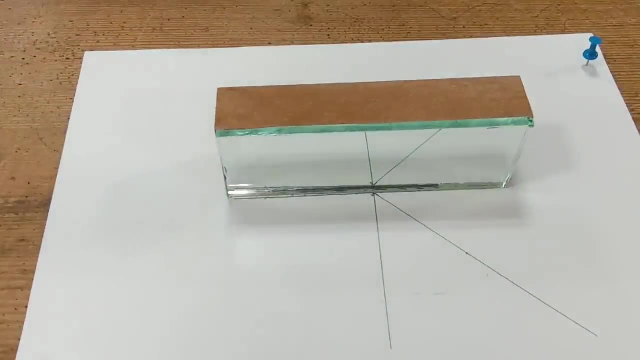 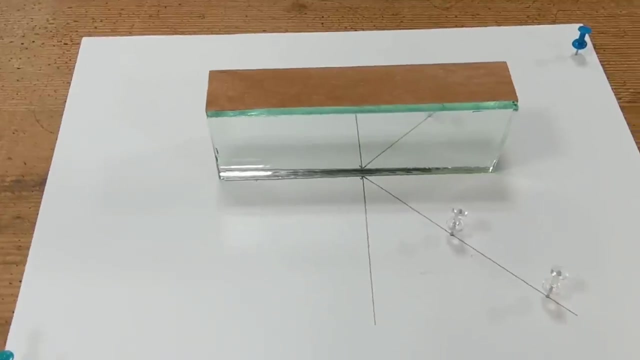 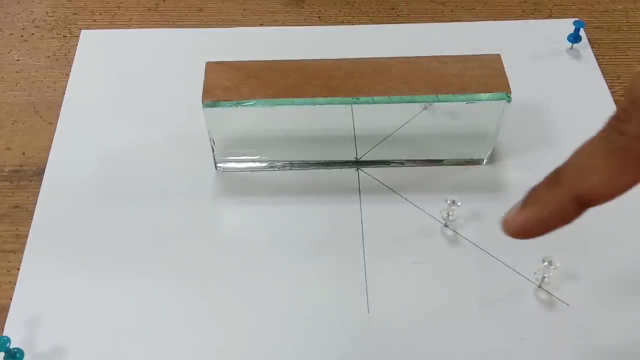 like this one. This is my incident ray. Now I am going to put the mirror here, and out of 4 soft board pins, I would be fixing 2 pins over here. Now, see guys, the image of these two pins will be visible in the mirror on the back side. Correct? So you will have two images of these two. 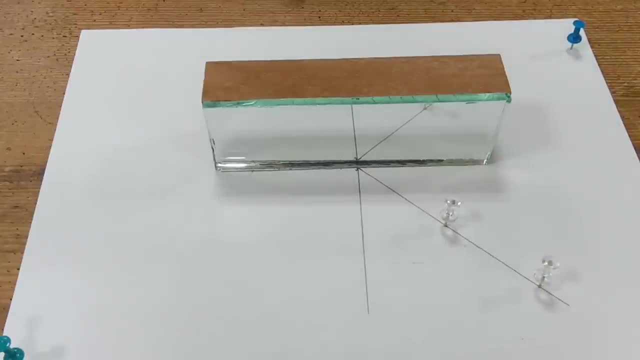 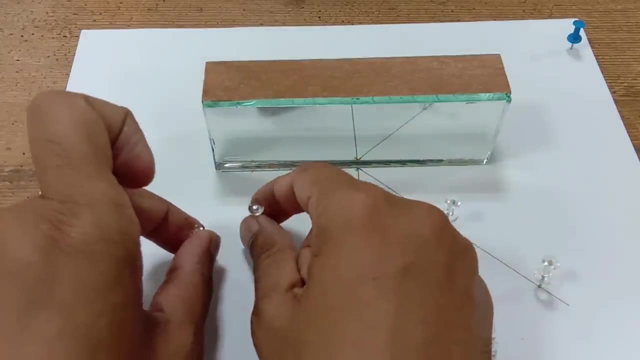 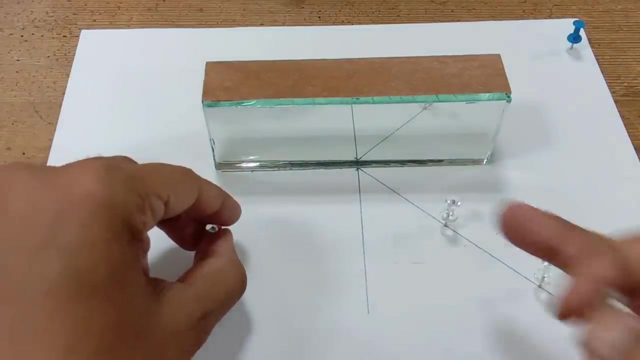 pins over here. Now, what am I going to do is I am going to take another two pins and I am going to arrange these two pins somewhere over here such that all four pins- two real pins and the other two images- appear in straight line, Right? So these two pins, their images, and these two pins, so all four. 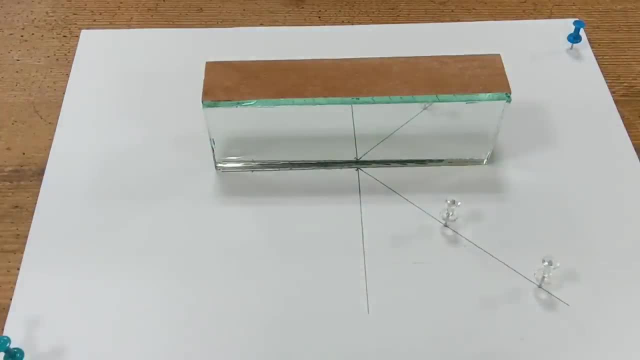 appear to be in straight line, So let me show it to you. Ok, I have arranged them So as you can see that these two kids, I have plugged it over here. Now let me show you. as you can see, the images of these two pins can be seen over here. 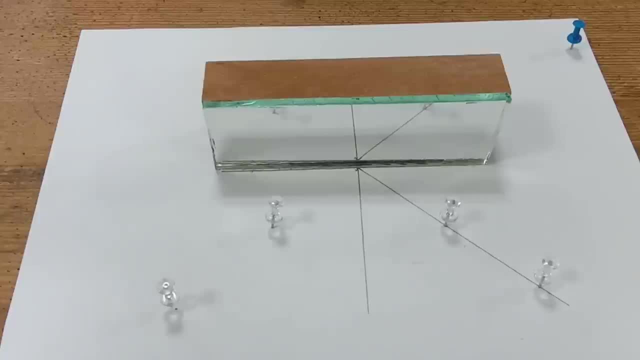 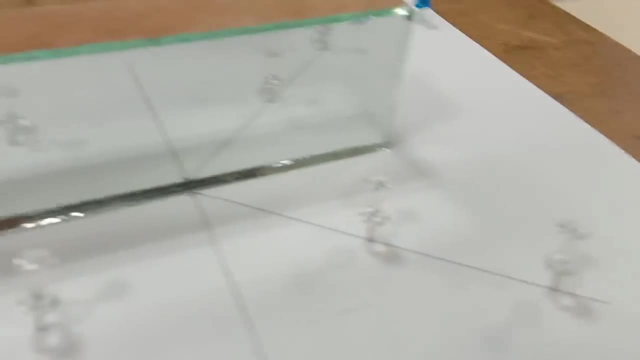 I have change the 240 degree angle. I can adjust it at 0 degrees of the back side. So I will just move this as I go over and stick this. So I am진 do this. saw the line Just like that. it becomes straight line. This is my incident ray. it is not fixed due to any sound. This is my incident ray, so it becomes straight line. All theseerna rays are one tangible field. there are five OHm, so one of these are two sebagai n przez these, each one, you can see the sixohm pickaxe which is visible when you turn off the lights. As an insertor. as an insertor, the highly wind, wind is seeds continue, sits here. 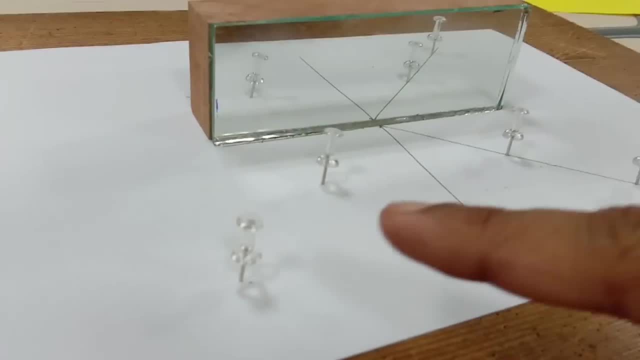 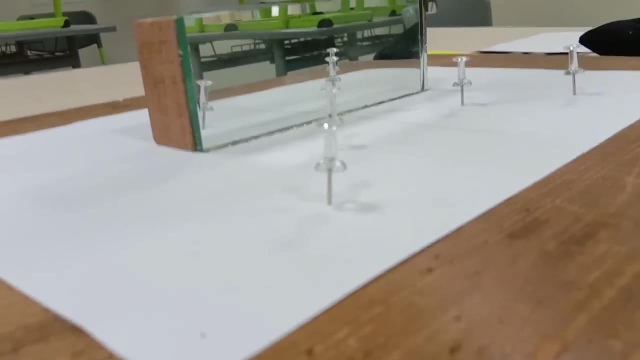 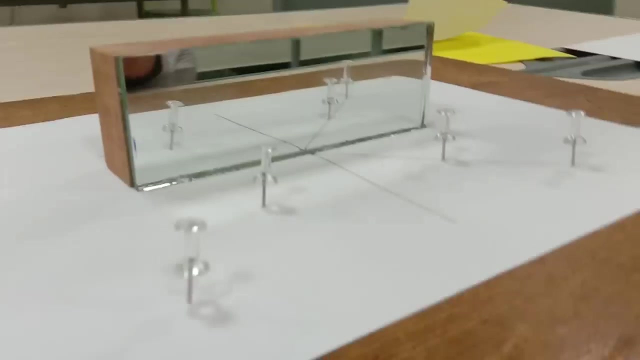 here like this: now, these two pins that I have plugged it over here as you can see that they all four pins are in straight line, right, these two pins- their images you can see there- and these two pins I have attached such that all four appear in straight line. now let me put back.